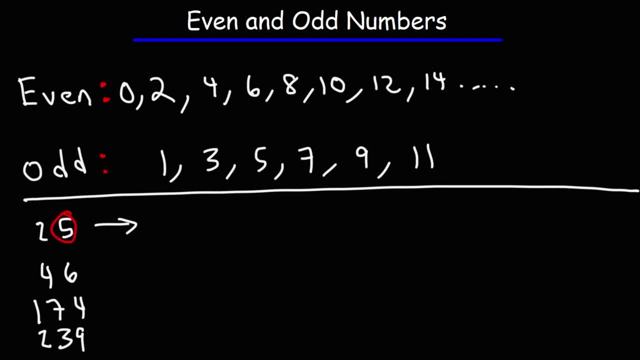 the one's digit, 5.. 5 is an odd number, So 25 is going to be odd. Now, what about 46?? So, looking at the last digit here, 6 is even, So 46 is going to be an even number: 174.. 4 is even, So 174 is an even number. 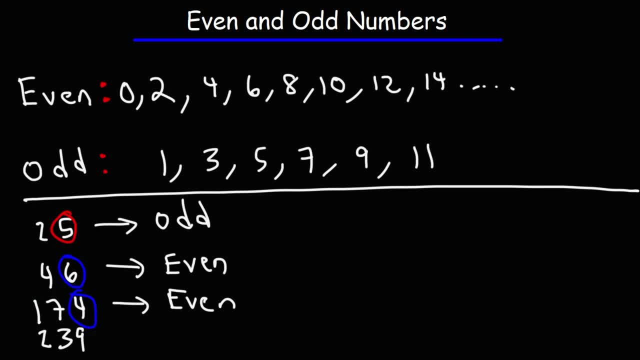 Both 46 and 174,. they're divisible by 2.. Any number from which you could divide by 2 and get an integer. As a result, it's going to be an even number. 2 doesn't go into 239, so that's not going to be even. 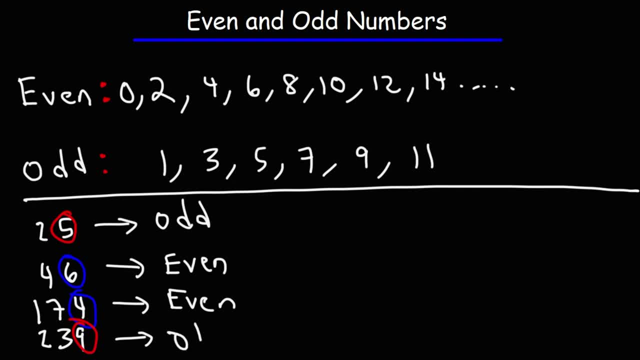 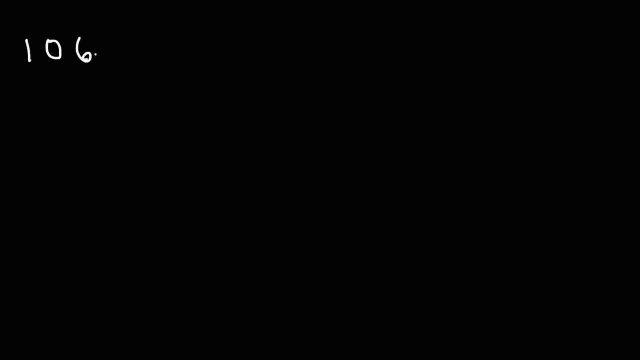 And the fact that if we look at 9,, 9 is an odd number, so 239 is going to be an odd number. Let's work on some other examples. Try these numbers: 1,067, 5,830,. 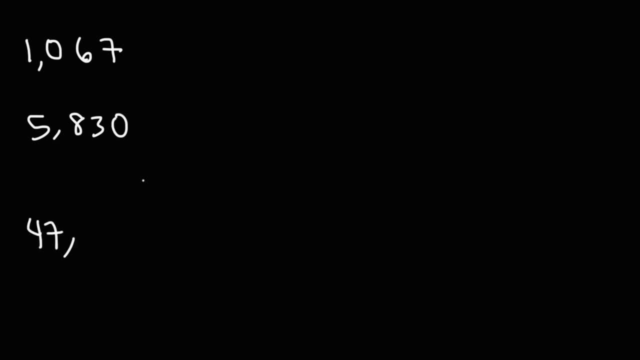 5,830, and 47,531.. So 1,067,. if we look at the last number, that number is odd, So the entire number will be odd: 58,030,. this ends in a 0.. 0 is even so. 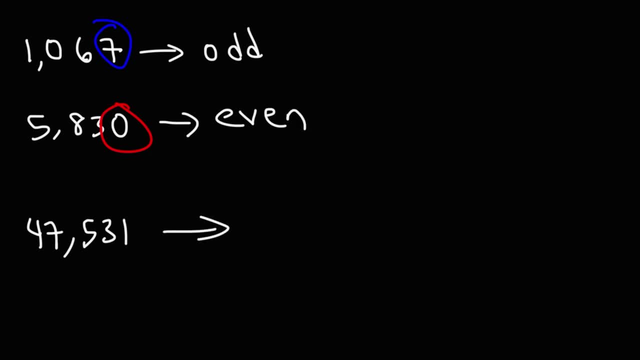 58,030 will be even. 47,531, 1 is odd, so that whole number is going to be odd. So that's a quick and simple way in which you can identify even and odd numbers. Now let's focus on operations of these numbers. 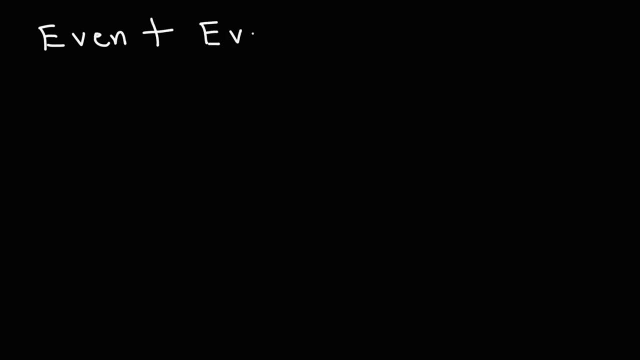 What happens when you add an even number with another even number? Will you get an even number or an odd number? The sum of two even numbers is an even number. For instance, if we were to add 4 and 8,, both are even numbers. 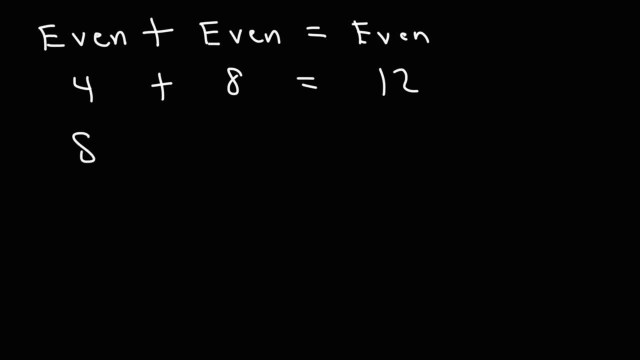 the result will be even: 8 plus 10 is 18, another even number, 132,, which is even plus 204, that's even. When you add up those numbers, you're going to get 336, which is even as well. 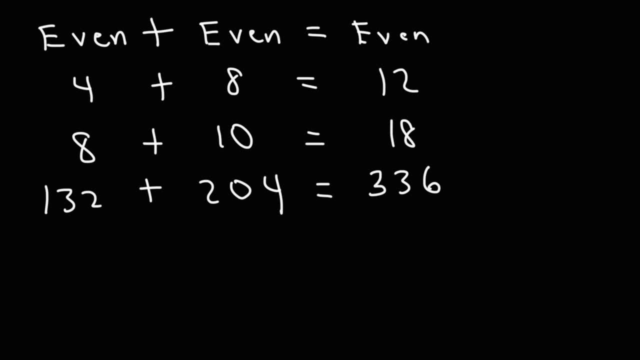 So the sum of two even numbers will give you an even result. Now what happens when we add two odd numbers? An odd number plus an odd number will give you an even number. 5 plus 3, those are two odd numbers- is equal to 8.. 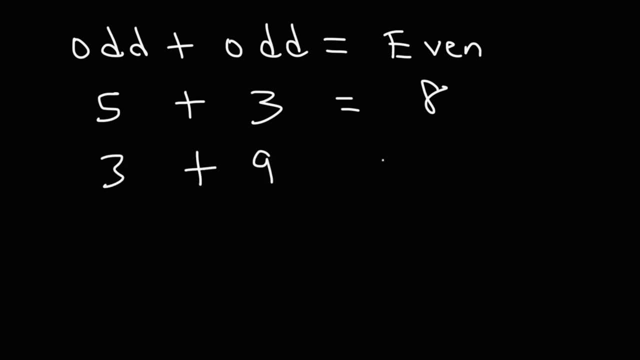 3 plus 9,. another set of two odd numbers that is 12.. 12 is even 13 plus 19,. that's going to be 32, another even number: 7, plus 11,. two odd numbers will give you an even result: 18.. 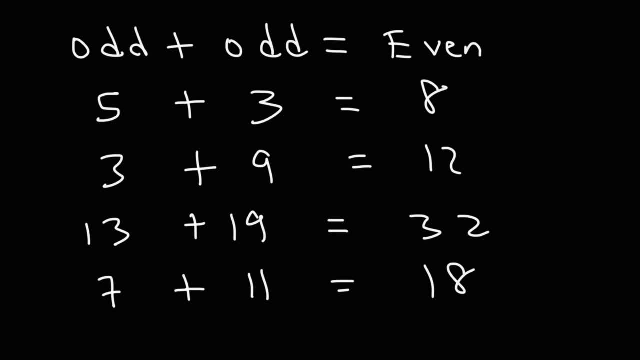 So the sum of two odd numbers is an even number and the sum of two even numbers is also an even number. Now what if we add an even number and an odd number? When you add these two, the result will be odd. 2 is an even number, 3 is an odd number. 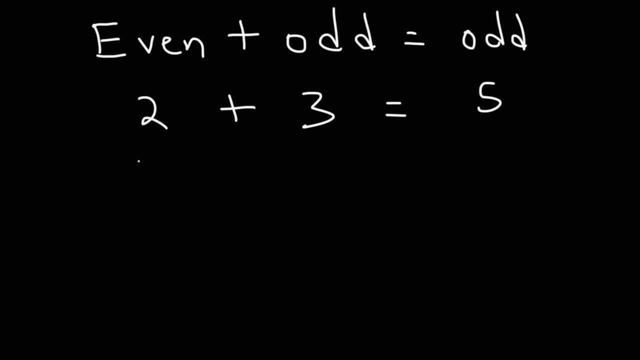 2 plus 3 is 5,, that's odd. 4 is even 7 is odd. 4 plus 7 is 11,, which is also odd. And here we have 8 plus 9.. 8 plus 9 is 17,, which is odd. 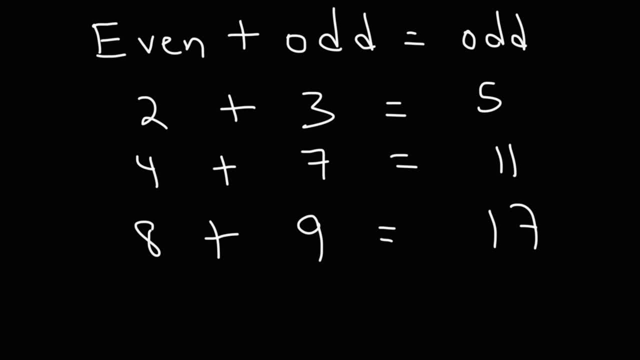 So anytime you add an even number with an odd number, you're going to get an odd result or an odd number. Now let's consider some other situations. What happens if we were to multiply an even number with another even number? What result do you think we're going to get? 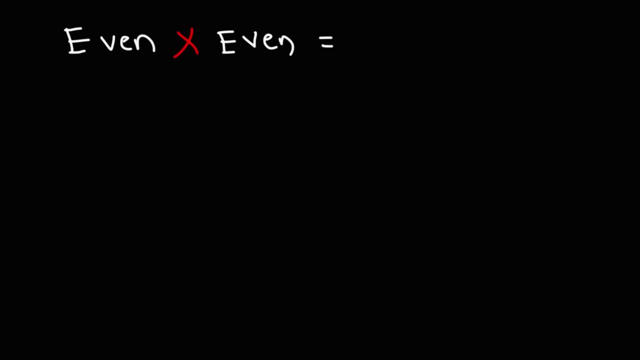 What's your guess on this one? An even number times an even number gives you an even number. So let's look at some examples. If we multiply 4 and 8, this will give us 32.. 6 is an even number. 12 is an even number. 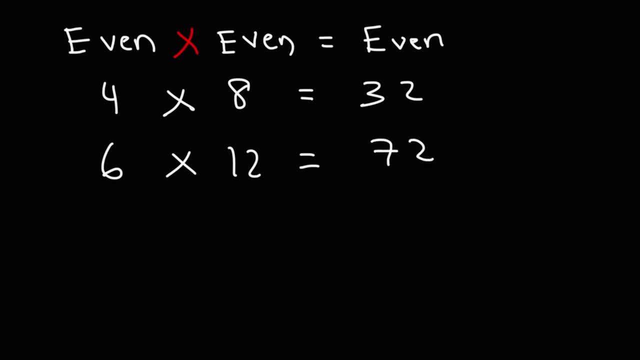 6 times 12 is 72.. Now what about 2 times 6?? 2 times 6 is 12, that's also even So. anytime you multiply an even number by an even number, you're going to get an even result. 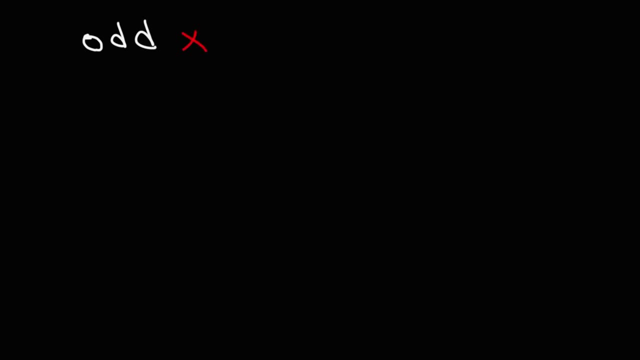 Now what's going to happen if we multiply an odd number with another odd number? So 3 is odd, and the same is true for 5.. If we multiply 2 times 6,, if we multiply 3 and 5, it's going to give us 15.. 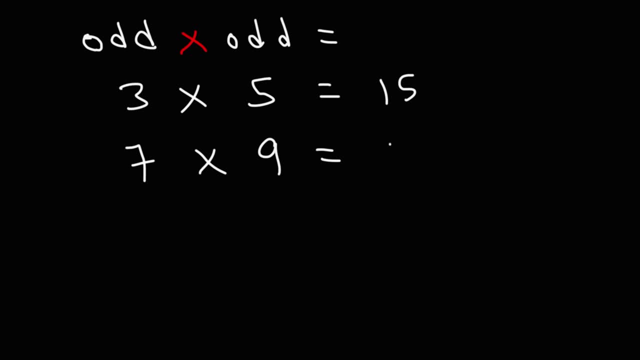 7 is odd, 9 is odd as well. 7 times 9,, that's 63.. Now let's try multiplying 11 by 13.. 11 times 13,, that's 143.. So we can see that whenever you multiply. 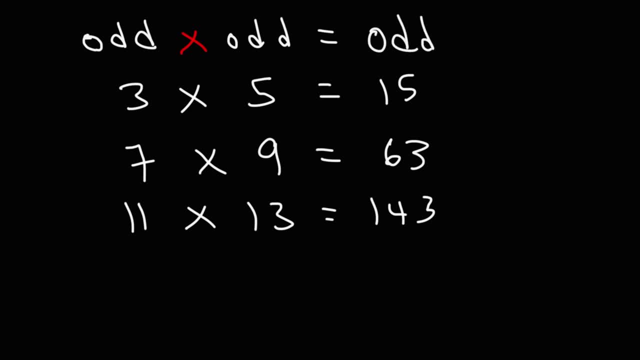 two odd numbers, you're going to get an odd result. So now what does that mean? What if we were to multiply an even and an odd number? What's going to happen? 2 is even. 3 is odd. 2 times 3 is 6, an even number. 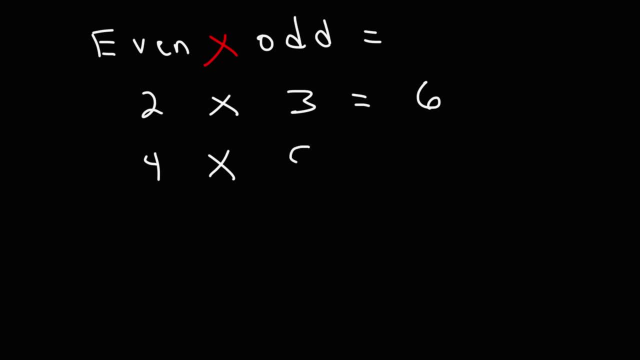 4 is even. 5 is odd. 4 times 5 is 20.. 8 is even 9 is odd. 8 times 9 is 72.. So an even number times an odd number will give you an even result. 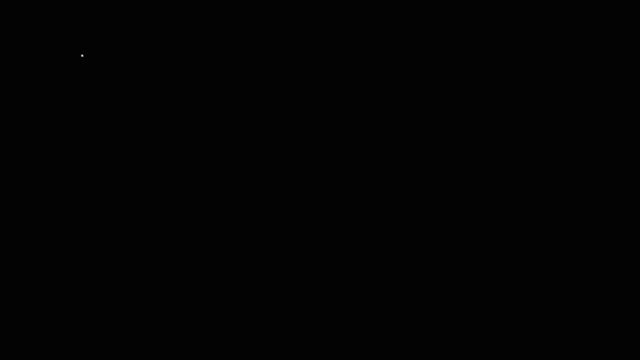 Now, what about subtraction? What happens if we were to subtract an even number with another even number? Let's say, if we take a large even number and subtract it by a small even number: 10 minus 4 is 6.. 18 minus 6 is 12.. 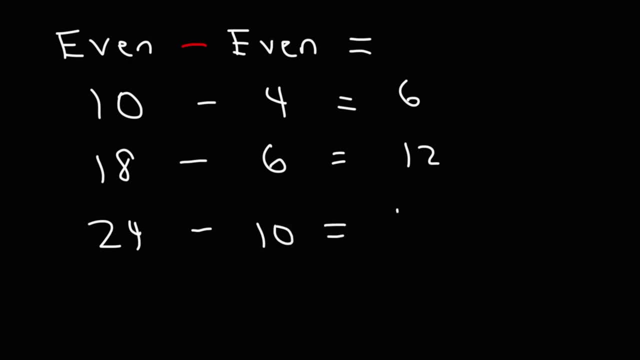 24 minus 10 is 14.. So any time you subtract an even number with another even number, you're going to get an even result. This is the reverse of adding two odd numbers, which gave us an even result. Now, when adding two odd numbers, we got an even number. 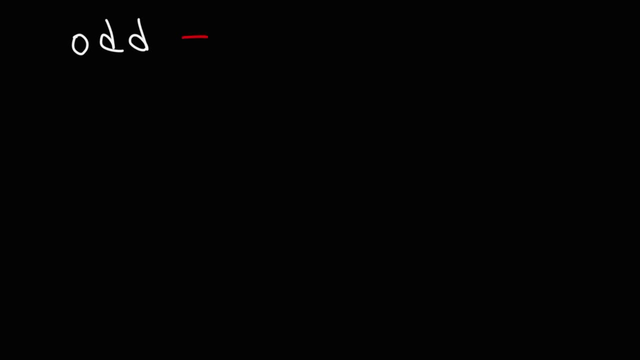 Let's see what's going to happen if we subtract two odd numbers. So let's take a large odd number and subtract it by a small odd number: 13 minus 7 is 6.. 17 minus 9 is 8..